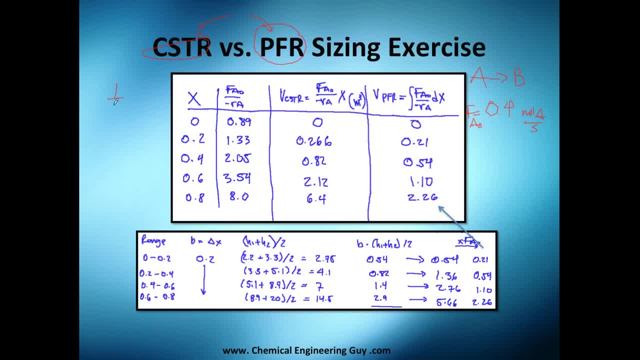 think it's everything, and we got the table with a rate of reactions versus conversion. now I'm substituting everything here. I got these conversions right here. I calculated this number here divided by the rate of reaction, which gave me these numbers, and I'm going to calculate the volumes involved in CSTR. 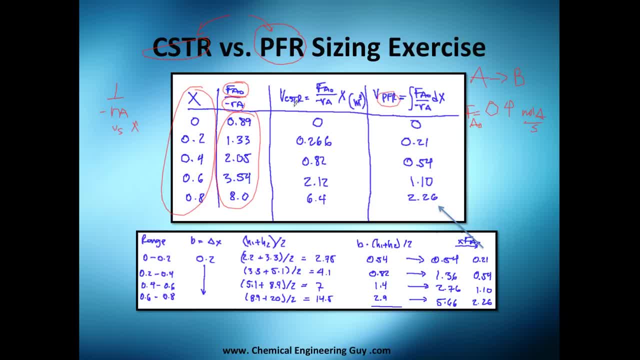 and the volumes of PFOR. so the ones of CSTR are very easy because they are once again done algebraically. so I got this value and I got this value, which is this column right here and this one here, and yeah, essentially, this time this 0, this time this gives me this and so on. so I got. 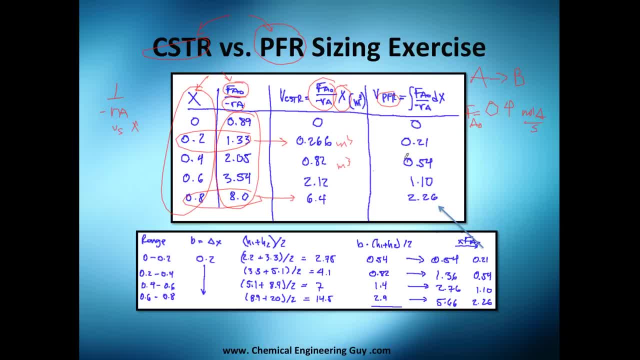 the volumes of CSTRs. now the interesting part comes into the PFOR. these are integrals. so once again I pop up this table I just done in the PFOR problem and I got these volumes here, volumes here, volumes here and volumes here. so I just 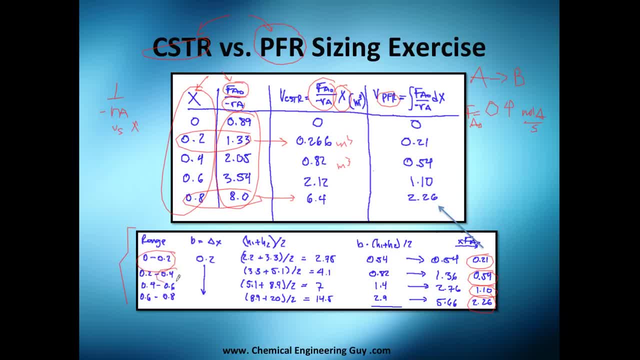 made sure that they are correctly assigned. this is for 20%, this is for 40%, this is for 6% and this is for 8%. so, and of course, 0 is 0, so I just drop them here and, yeah, they make sense. they are similar and typically as the 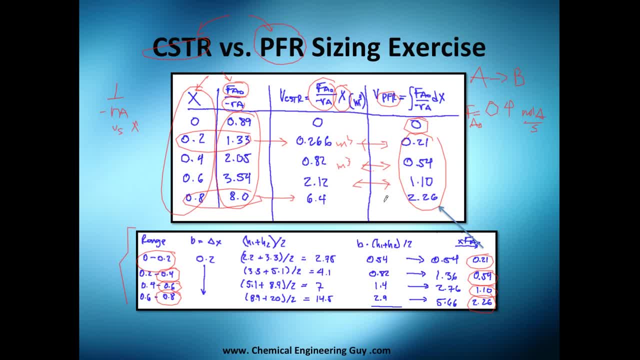 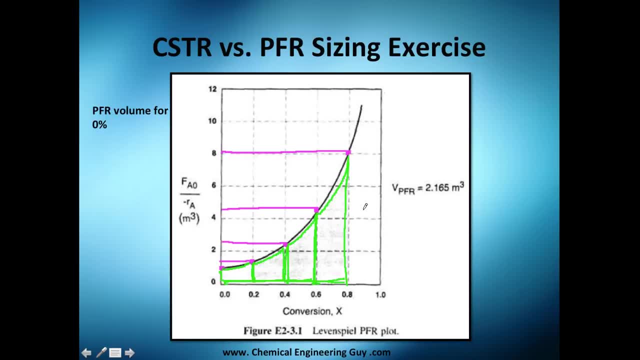 PFOR, given this rate of reaction, is a little bit less. so, yes, let's continue. let's do it more graphically, because numbers I like them a lot, but graphics are everything. so let's say PFOR at the conversion of 0%, well, you have nothing. 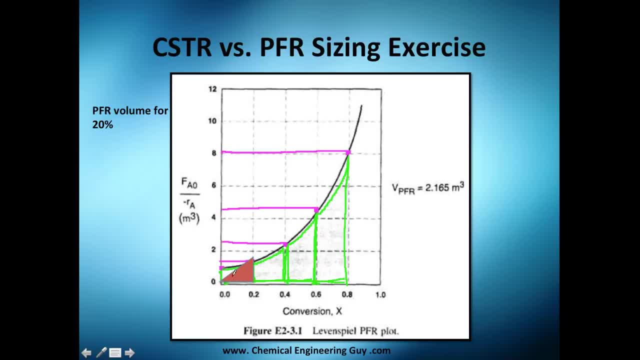 then at 20%, you get this area here. you should also include this. this will be a 20%. now include it. make it bigger: 40%, 60%, 80%. that's the total volume of PFOR. if you were to calculate the volumes, you will only calculate, though, that area. 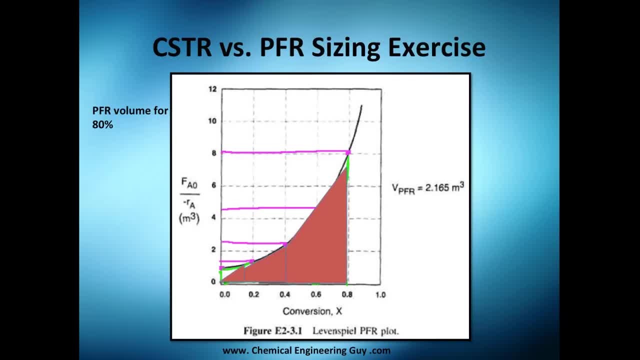 very nice. okay, now let's calculate the CSTRs. so for a 0% conversion, you will have no volume. for a 20% conversion, you will have that volume. for a 40% increases, and then it still is a rectangle and the 80% rule goes up, so of 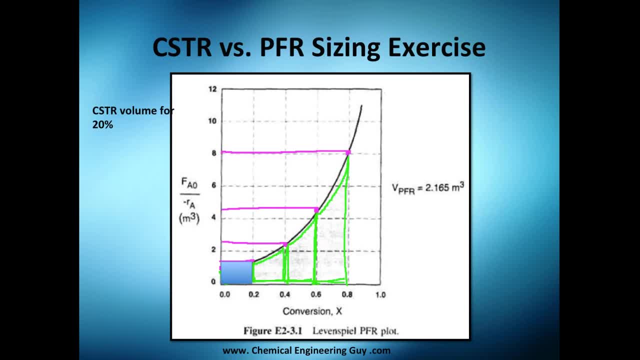 course, sorry about that. if you compare these volumes, you always have an excess. so, for example, this part right here is the excess. this part right here is an excess, this part right here, it's also an excess. and, as you can see, obviously this part actually I I don't even know if I'm right for drawing it, but this is also an excess. 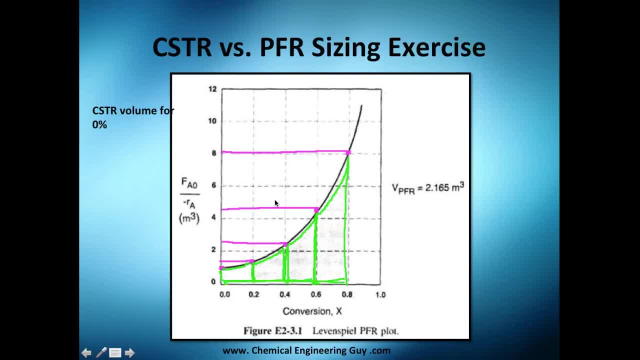 and why? why is it so? because of the rate of reaction or the shape it takes. so just take care, you will have a different shape of reaction like someone like this. you will have lower rate, of lower volumes for CSTR and higher volumes for PFOR. but this is. 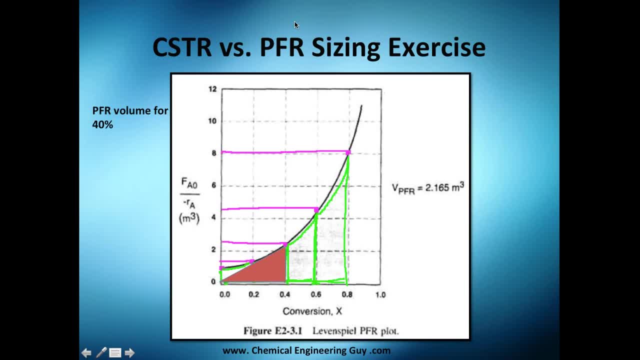 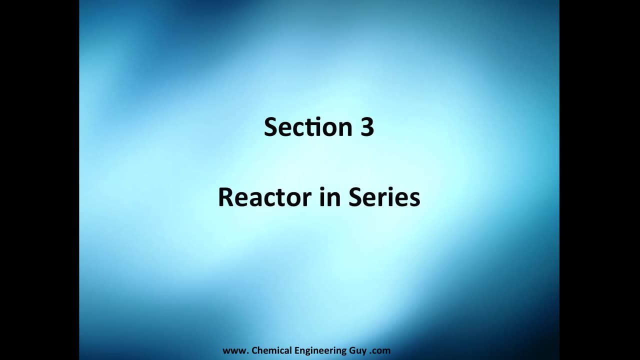 not the case, and I just wanted to show you how the area under the curve in this case is lower than the rectangle of these ones and I, as you can see, we have stumbled upon these slides. we are done with this section number two, and we will continue with section three, which is essentially 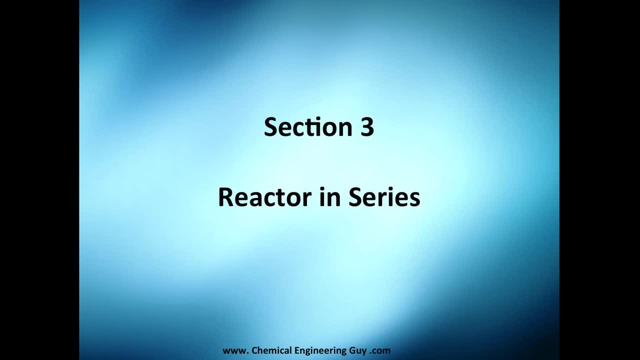 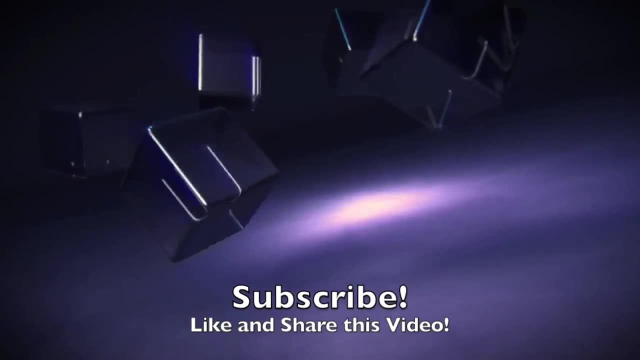 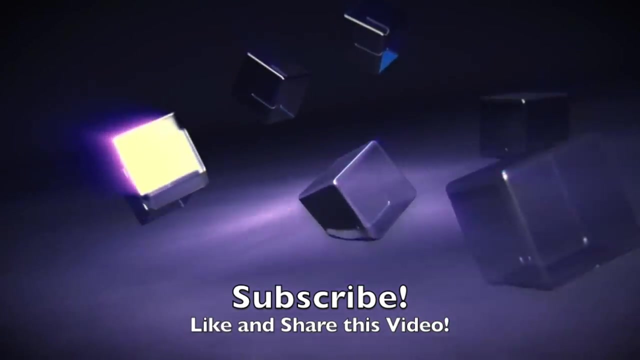 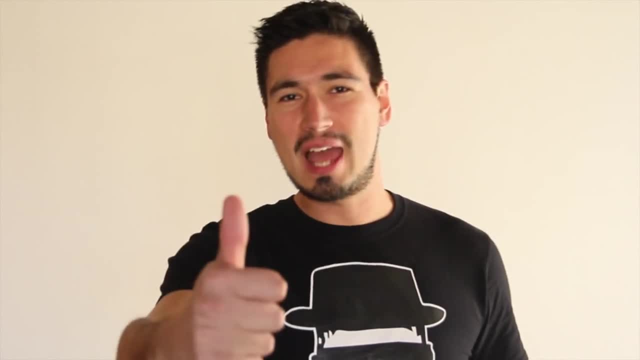 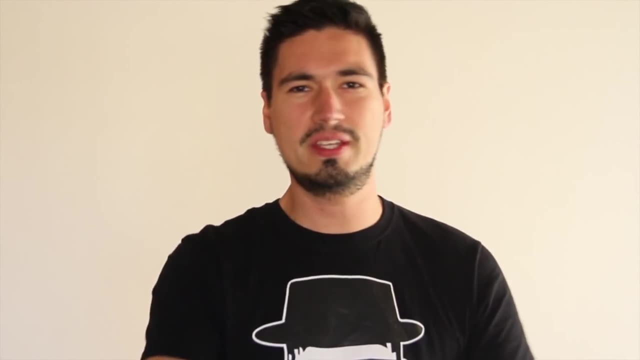 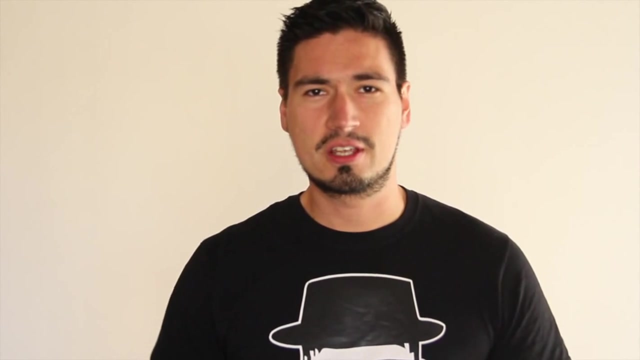 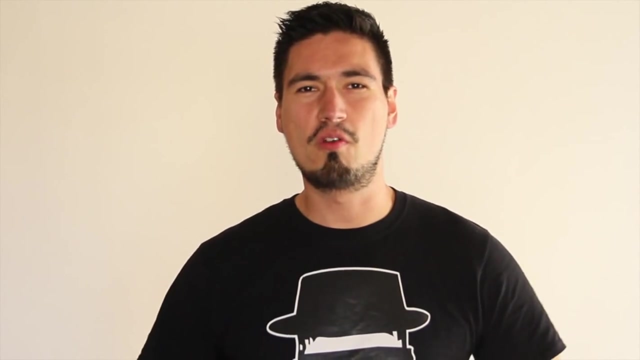 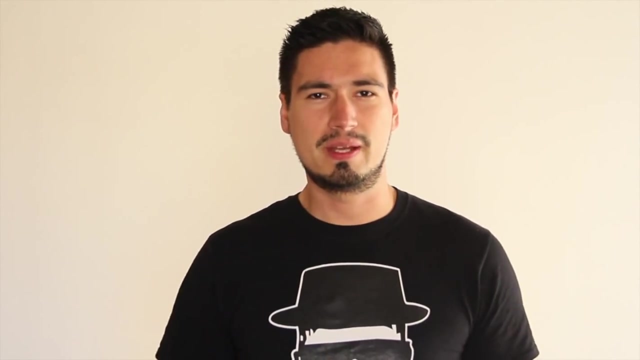 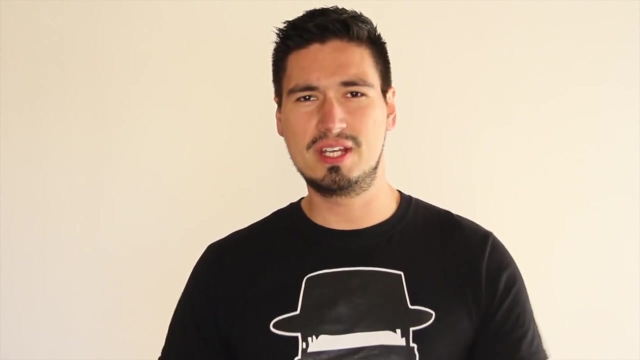 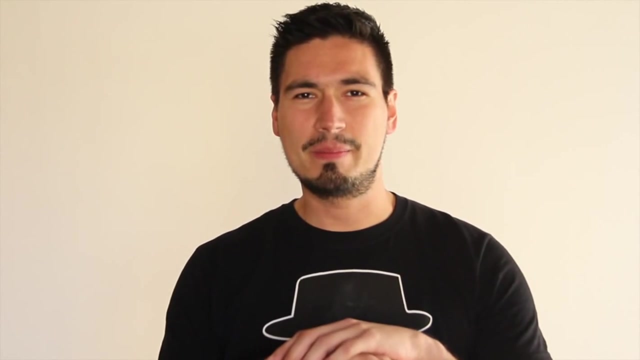 bye, bye. Uploads, experiments, playlists, whatever content I'm getting on YouTube, be sure to click the subscribe button. Subscribing to the channel is totally free, guys. My dream is to create an online academy of chemical engineering where everyone can access it in the world. 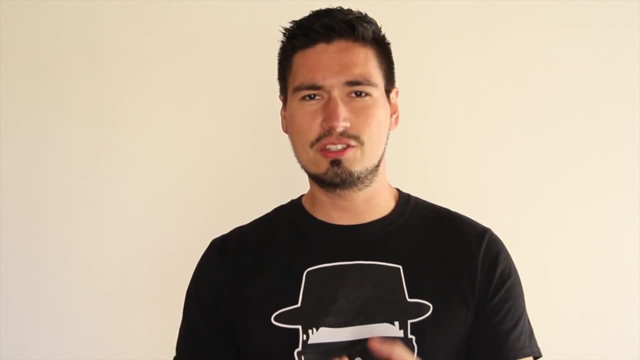 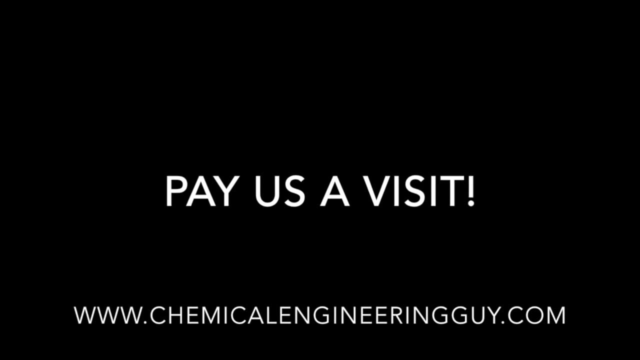 Imagine a place in which the student, the teacher and the engineer get the best of each other. Thank you, thank you, thank you, guys, for the support and the love. 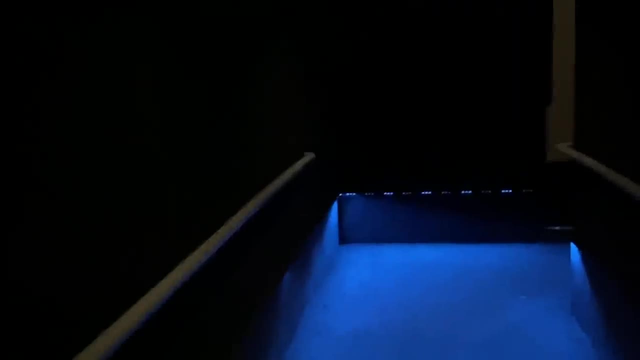 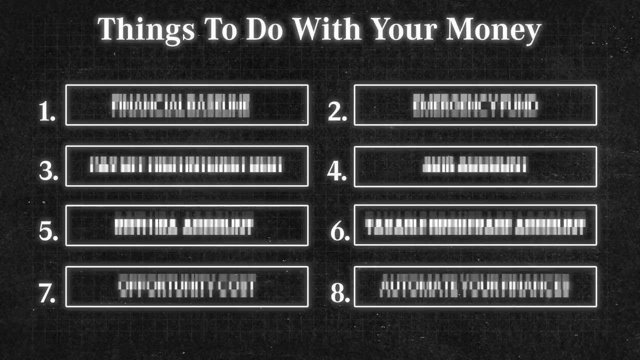 It's Friday, just got paid New shoes, new restaurant movies and it's gone. When it comes to payday, it's hard to know the best things to do with your money. So today I'm going through, step by step, the 8 things you need to do with your money. 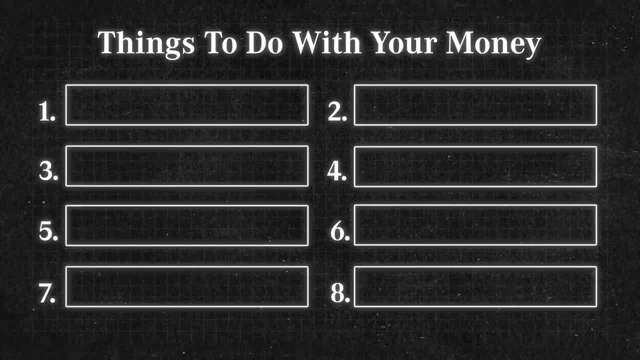 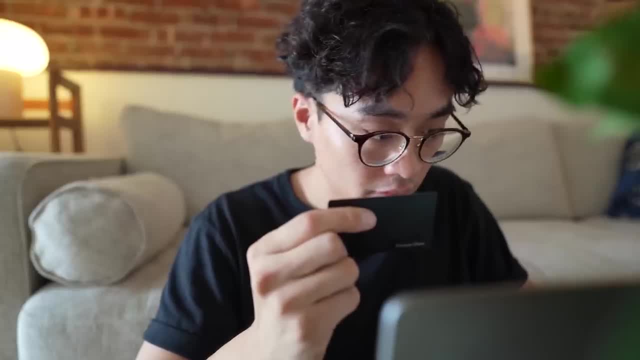 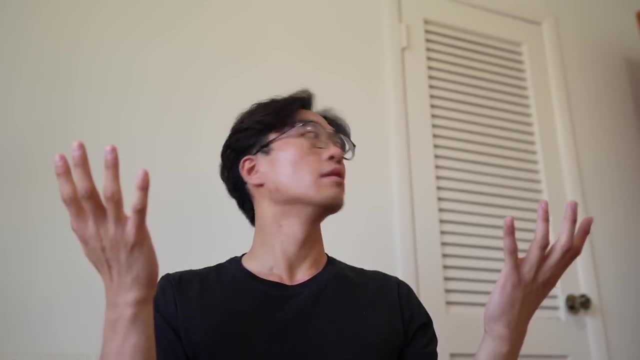 as soon as you get paid, The first and most important thing you need to do is find your financial baseline. When it comes to personal finance, most people feel like it's too much work, But that's why most people struggle. 64% of Americans live paycheck to paycheck, because they commit one of the worst financial mistakes. 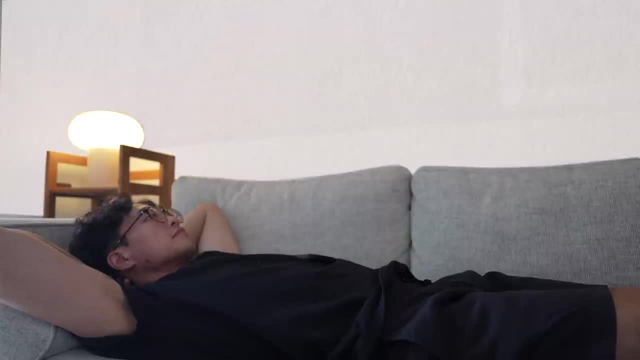 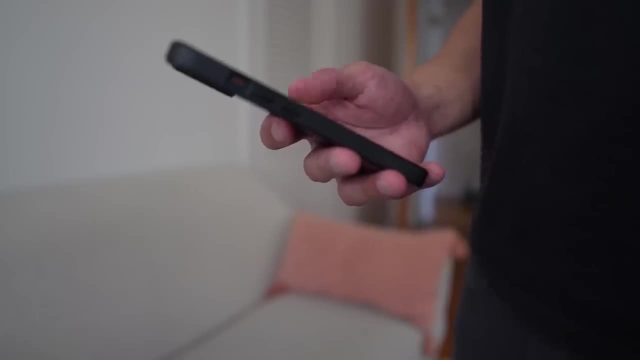 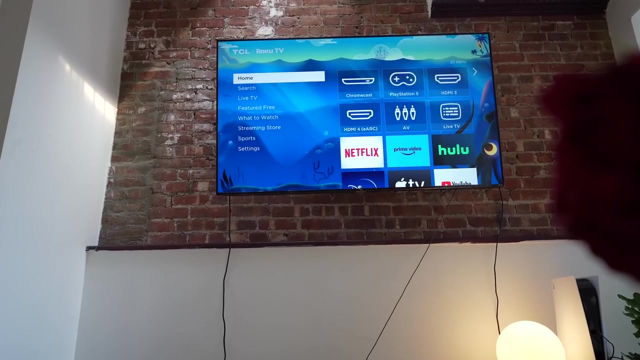 In psychology they call it mental accounting. Basically, it's when you mentally categorize your money instead of physically writing it down- In May you might receive a tax refund from the IRS- and you mentally categorize this as extra fund money. You get excited and start spending it: A new PS5, a new TV, or Mr Magic. 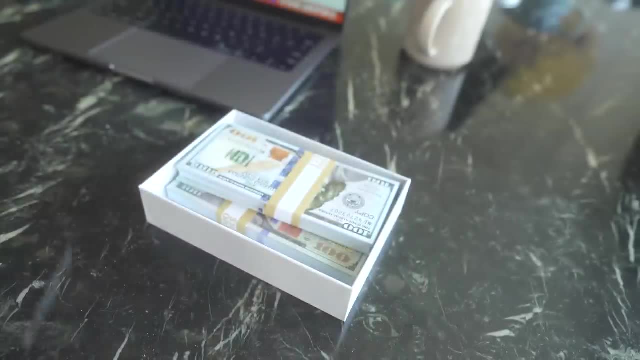 Lamp. The problem is this money is the same as your regular income. You just pay $2,000 a month and you get paid $1,000 a month. You get paid $2,000 a month and you get paid $2,000. $2,000 a month and you get paid $2,000 a month. You get paid $2,000 a month and you get paid $2,000 a month and you get paid $2,000 a month. You get paid $2,000 a month and you get paid $2,000.